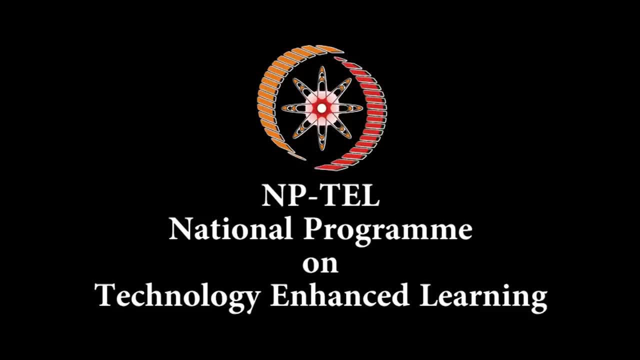 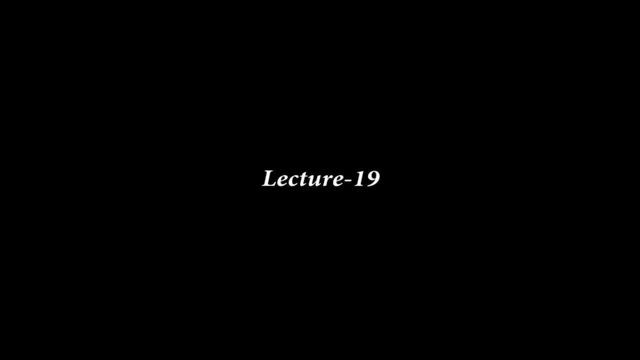 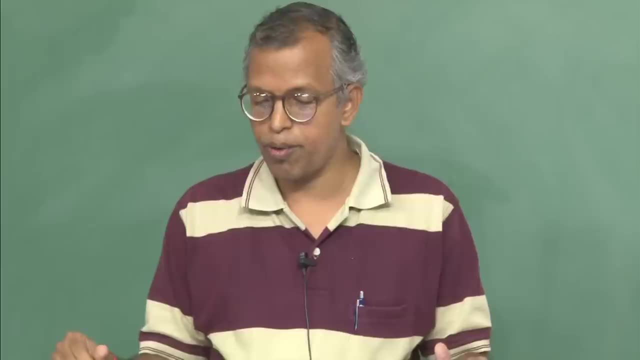 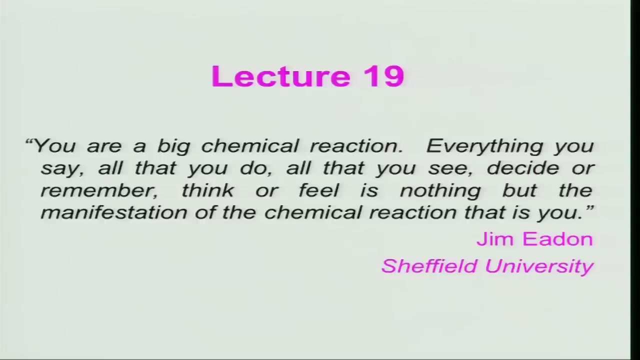 Let us start this lecture with a thought process from Jim Eden from Seafield University. He says that you are a big chemical reaction. Everything you say, all that you do, all that you see, decide or remember, think or feel is nothing but the manifestation of the chemical. 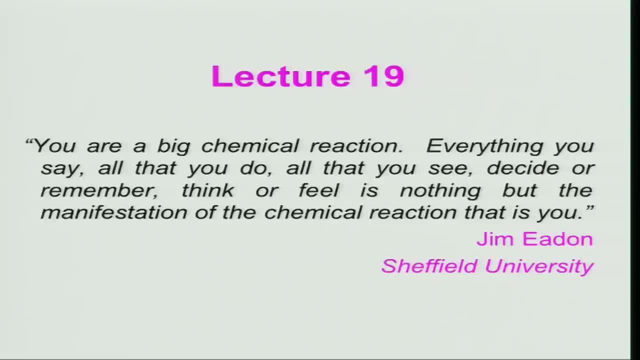 reaction. that is you. It is a very profound statement and I told you, nature does a lot of activities through us with the help of chemistry. That is the beauty of this, and let us recall briefly what we had learned in the last lecture. We basically discussed: 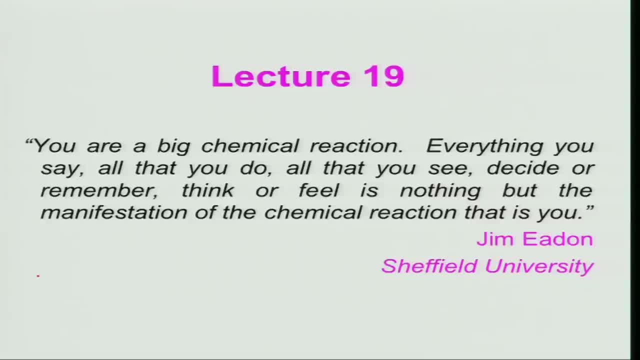 about Hayes law. and then we moved to how to find out adiabatic temperature. Then the adiabatic temperature: we found out that it is function of equivalence ratio, It is a function of inlet temperature, It is a function of also the pressure. Keep in mind that what 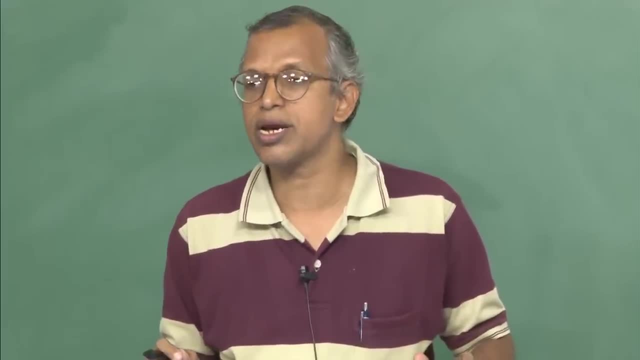 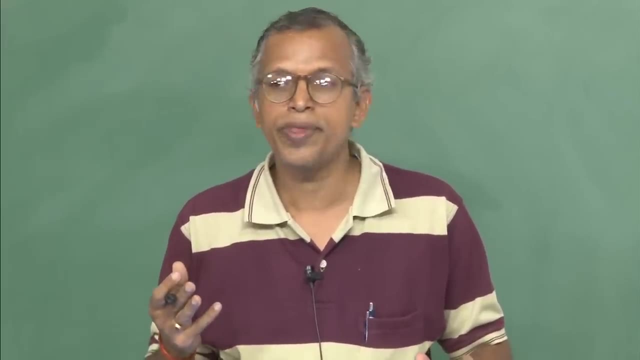 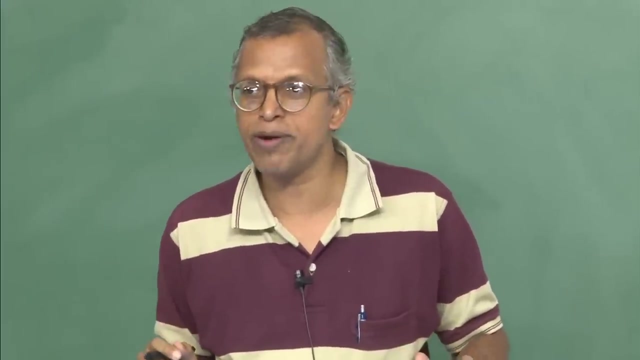 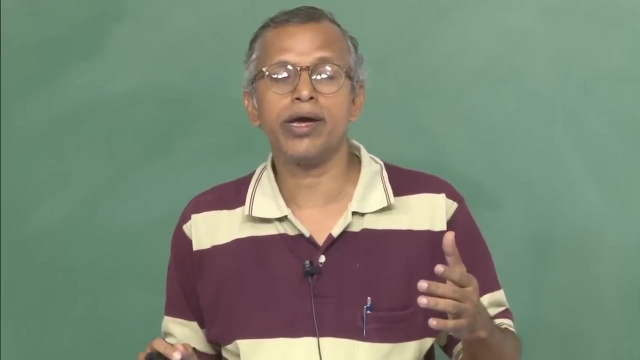 I had derived in the last class. That is mean for constant pressure process. However, some of the process occurs in the… the constant volume process. you need to think how we will have to find out adiabatic temperature for that, And remember that I did those things, keeping that you know this chemical composition. 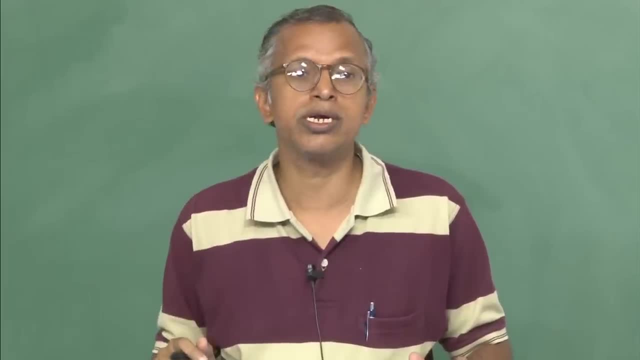 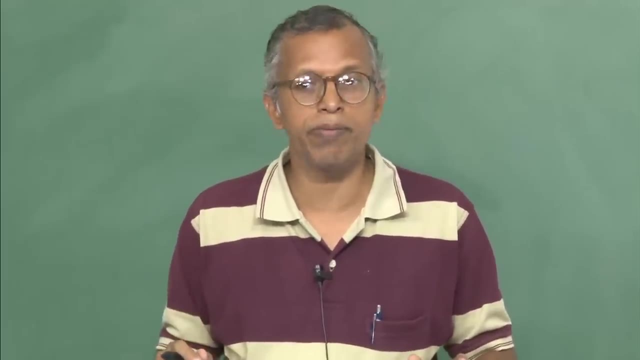 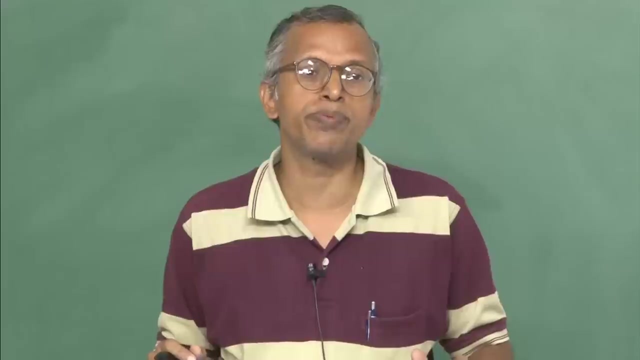 being known, but, however, in real situation chemical composition is not being known. and if both are interlinked, And then we moved into equilibrium, because from at equilibrium we can find out, we learn that the by minimization of the Gibbs free energy, we can find out the 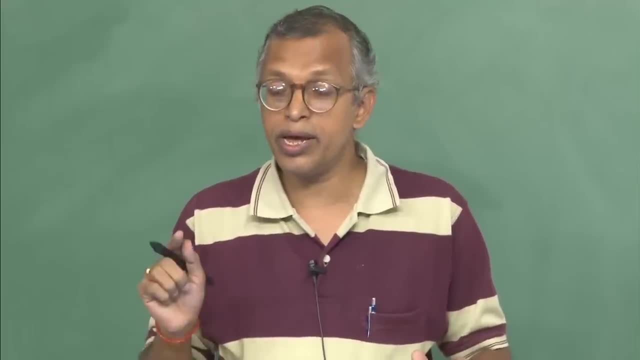 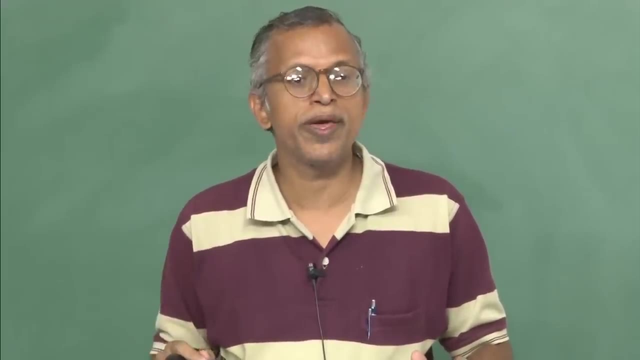 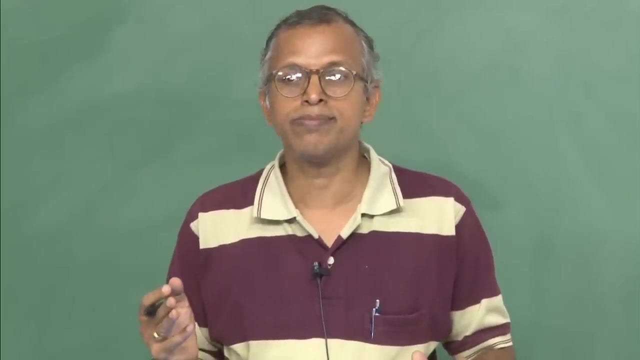 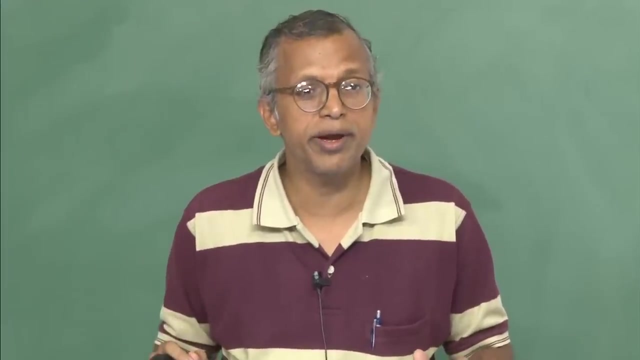 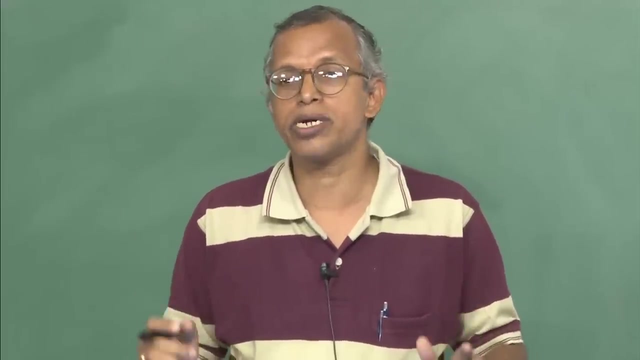 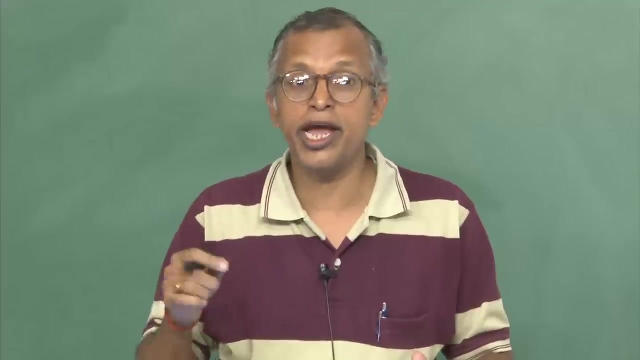 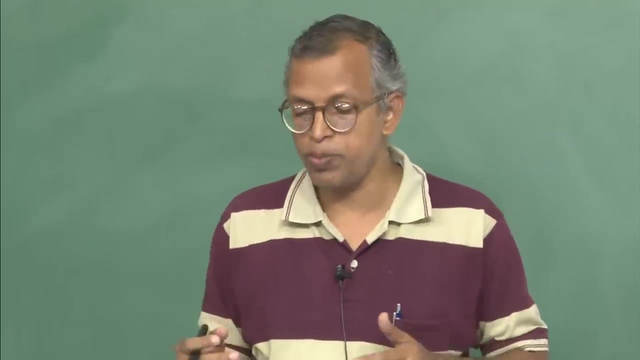 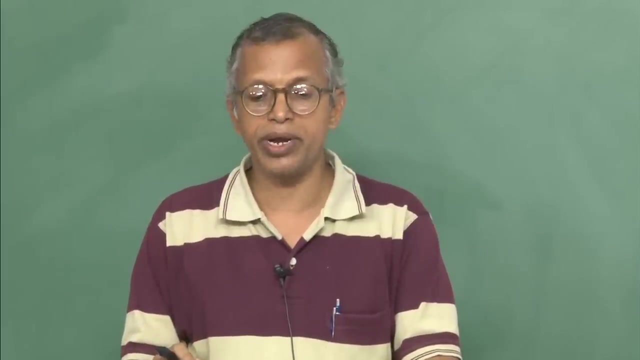 equilibrium composition right And keep. again I must draw your attention that this minimization of Gibbs free energy can be applied only for the control volume, So that you will have to look at it. I would not be covering, I will be concentrating on the minimization of Gibbs free energy. Let us look at how we will be dealing with it. 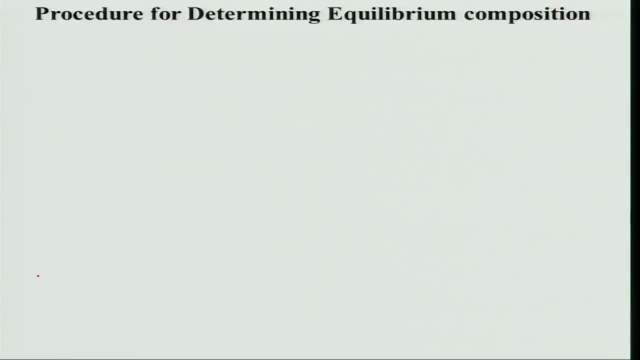 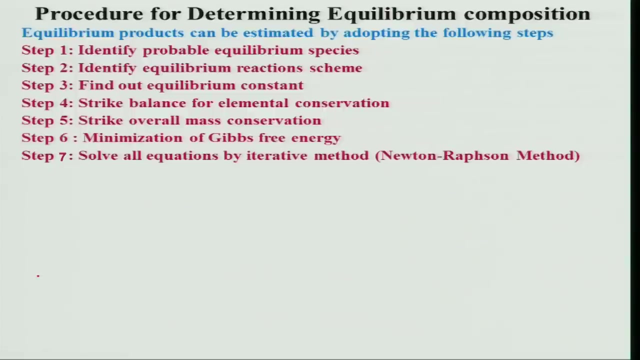 and, as I tell you, we will have to basically look at the procedure for determining the equilibrium compositions, And I have just identified few steps. of course, first of all, you know one has to look at what reaction it is. when you talk about reactions, You look to identify probable equilibrium species. You may ask a question how I will. 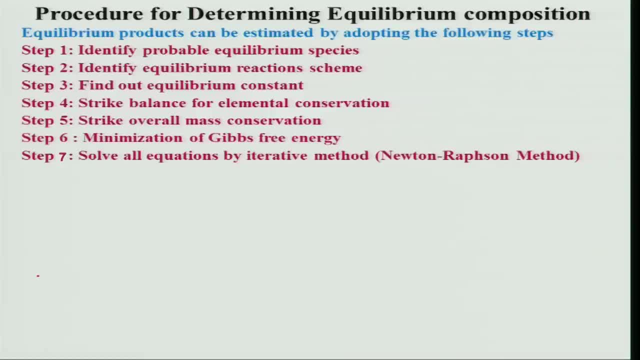 know that of course you need to have some experience And even if you choose something you know just by guessing, then you can figure it out at the end of this calculation whether it is of work doing that or not, Because the composition, if it is very, very less you know. 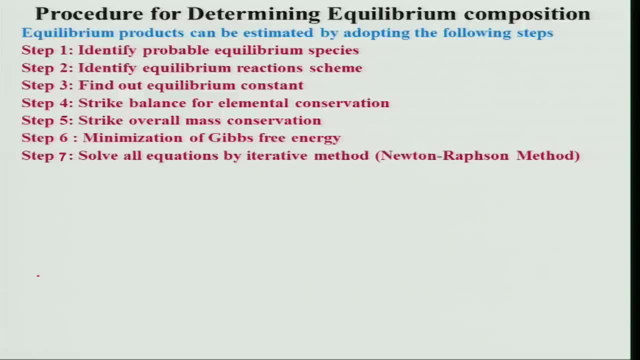 as compare to the major component. you can say, I can neglect it, but you will have to pay price for that because number of equations will be increasing. Then you need to what you call identify the equilibrium reaction scheme. that is also is a important aspect. what are they learn and? 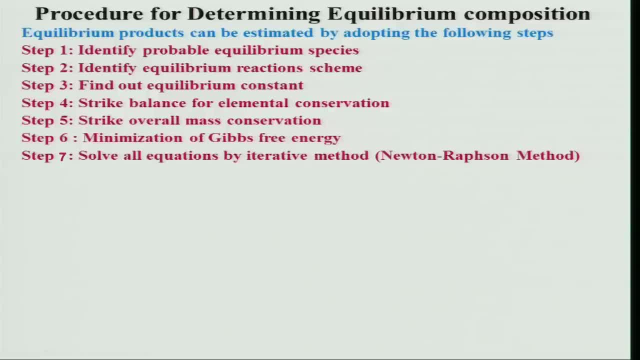 then these reactions must be elementary in nature. that is a very important point. Then you need to find out equilibrium constant. what is that equilibrium constant? some of you might be aware because it is being taught in the you know, your engineering and other things. So we need to determine that equilibrium constant, right. and then, of course, for that, 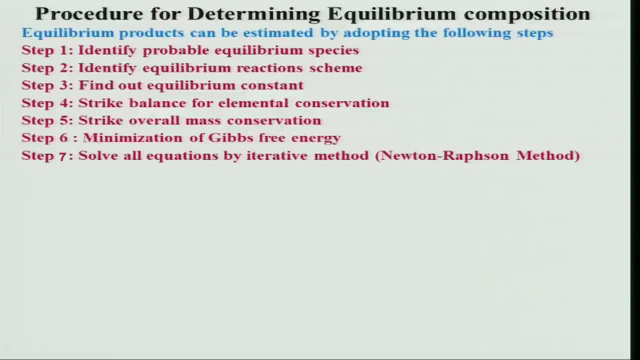 we will have to, for you know. next step would be strike a balance for elementary conservation, strike overall mass conservation and then minimization of Gibbs, free energy right And solve all equation, you know, by iterative method, Because all are coupled equations. So you cannot really solve like that, although it 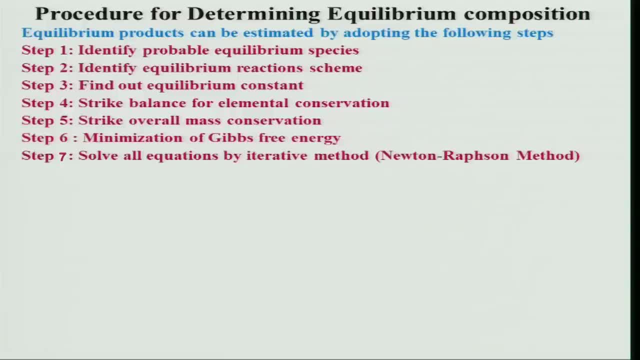 is algebraic but it will be, you know, coupled. So you need to use iterative method. one of the numerical tool which is being used is the Newton Raphson method for solving. So we will, as I told, we will be considering ideal gas mixture all the time So Gibbs function. 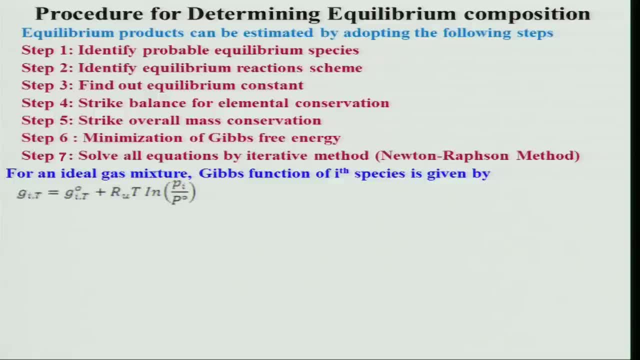 for I S spaces can be written as the G I T. that means this is the ideal gas mixture. the I S spaces Gibbs free energy at particular temperature, and this is at standard state. you know like temperature and pressure, And then plus R, u, T, l, n, P, i by P, naught you keep. 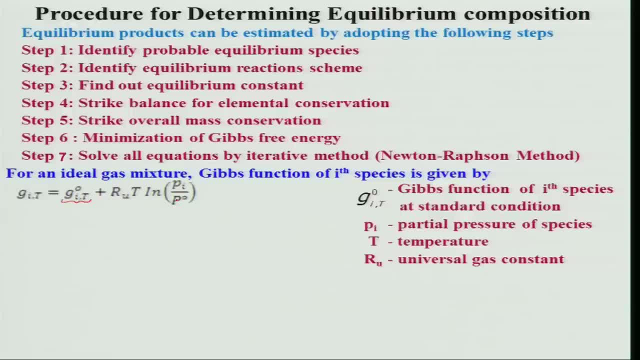 in mind that P, i is basically partial pressure of the I S spaces and T is the temperature. R? u is the universal gas constant right. That means this is: this is the ideal gas mixture. expression is mean for a particular spaces. it can be methane, it can be propane, it can. 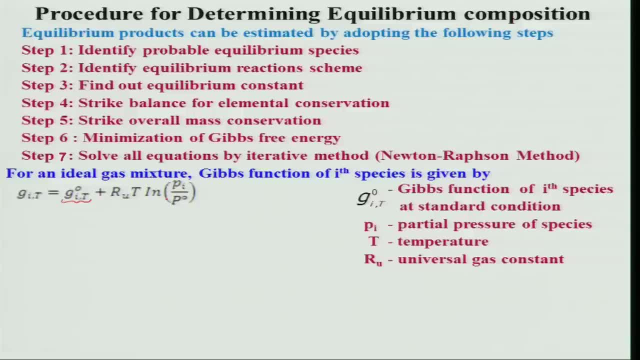 be oxygen, it can be O, H, any other things. So what it indicates, it depends on temperature. it depends on also partial pressure, and P naught is your what you call the standard pressure, in this case ambient pressure, which is being considered. So Gibbs function for an ideal gas mixture. we know that G mixture will be. summation of. 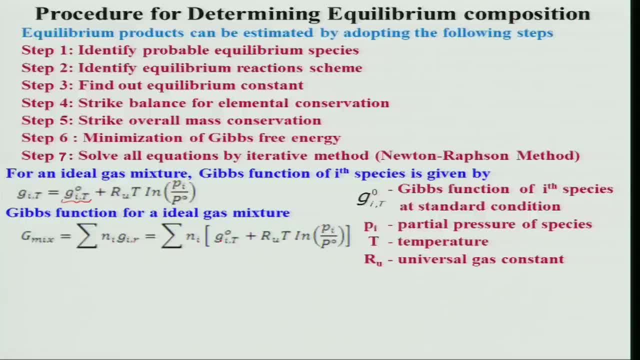 N? i, g i r And N? i into G I, T? R? u. you can just write down this expression over here. you know, if you look at, this expression can be put it over here. that is all, rather it. this expression can be put it here and you will get this thing. So what we will do now, we will have to basically.